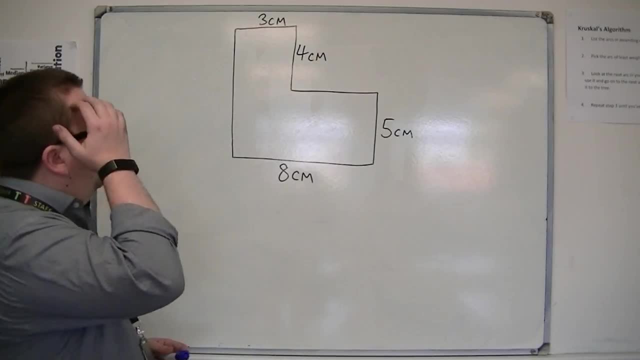 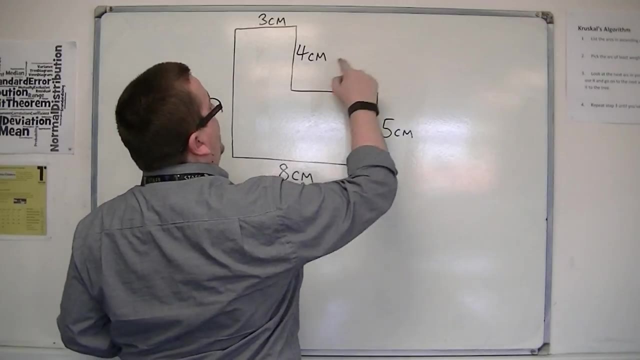 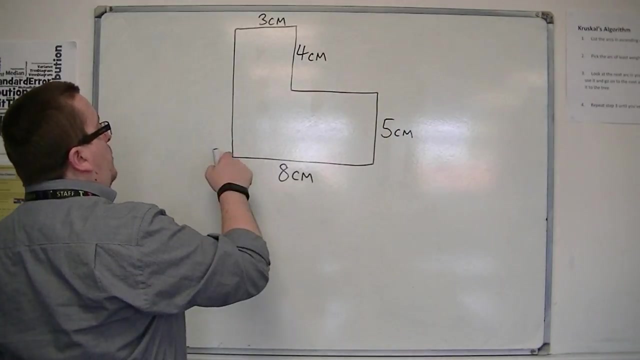 Because they may well come in useful. So if you know, for example, that this side is 5cm and then it goes up another 4cm, as it does there, Then the whole thing must be 9cm high, And so this length must be 9cm. 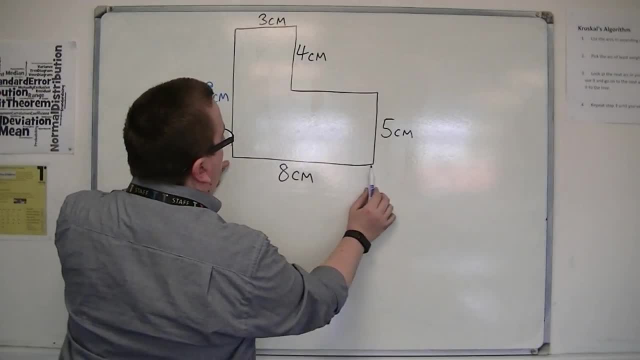 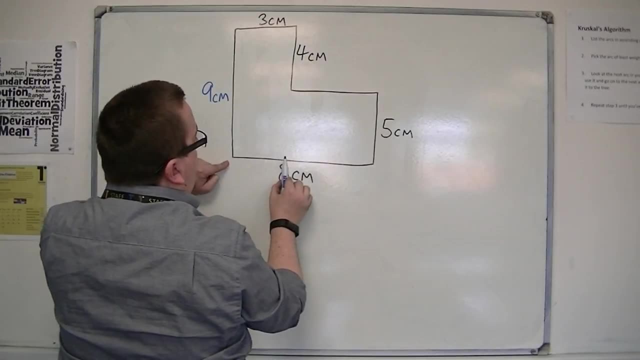 And likewise, if you know that the whole length of the shape is 8cm, But you know that that portion of it is 3cm, So we go all the way up to 3cm, and then what must be left is 5cm. 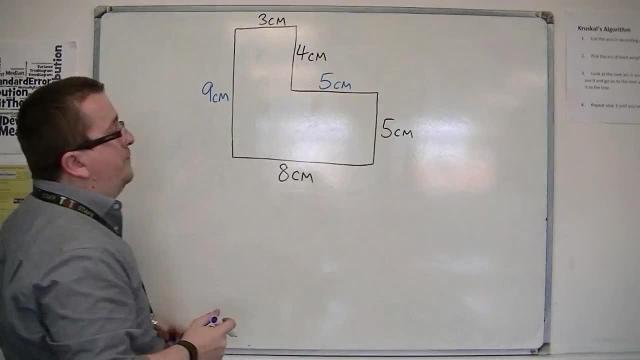 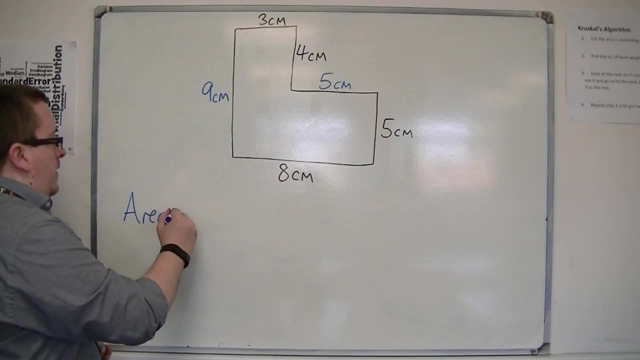 So this must be 5cm long This section. So once we've done that, If you're wanting to find The area, Then what you want to do is split the shape up into shapes that you know you can work the area out for. 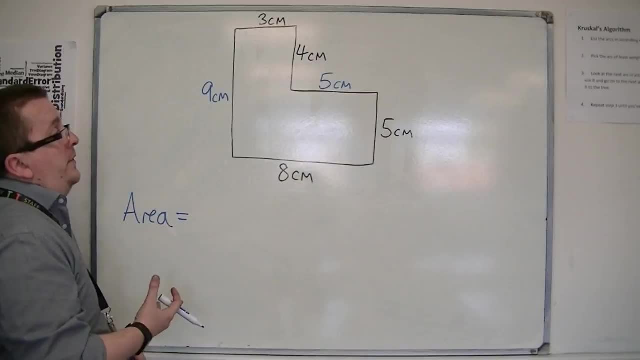 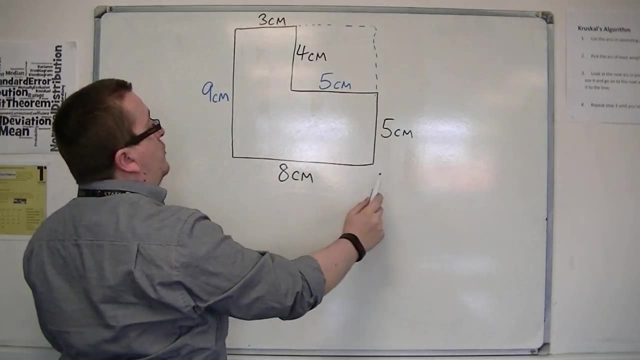 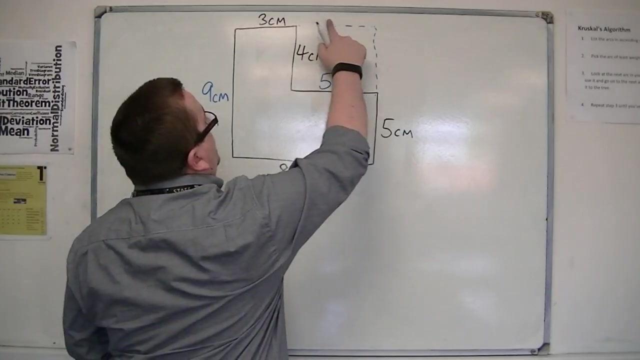 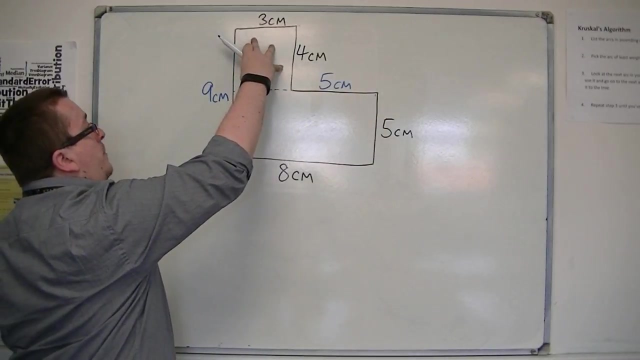 So you can split this in different ways. You could, for example, find the area of the whole shape and take away the area of that rectangle there. Or You might split the shape this way: Find out the area of that shape, Add it to the area of that shape. 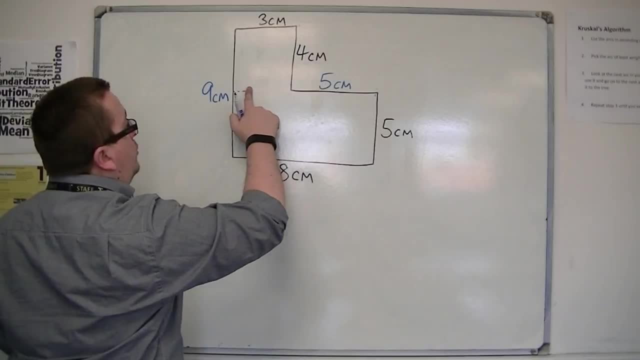 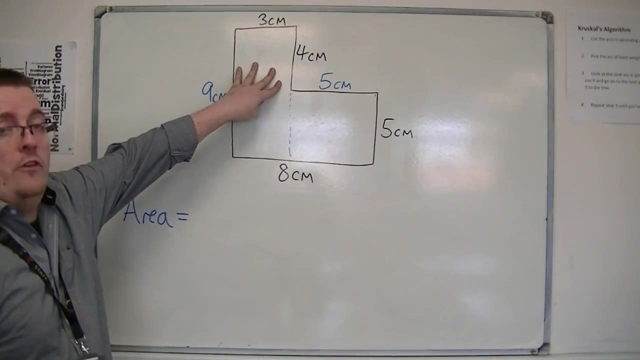 And then you've got the area of the whole shape. You could split it down this way: Okay, And do a similar area of this shape plus the area of that shape gets you the whole area. So whichever way round you do it, it doesn't matter. 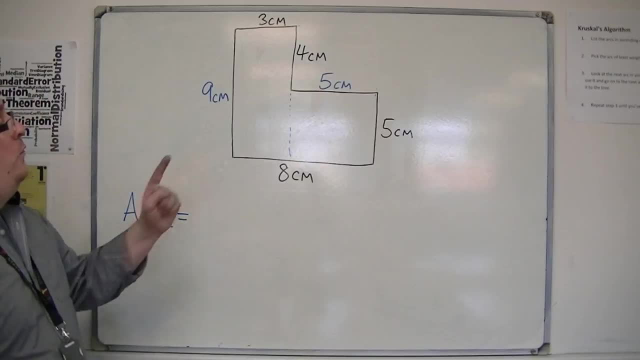 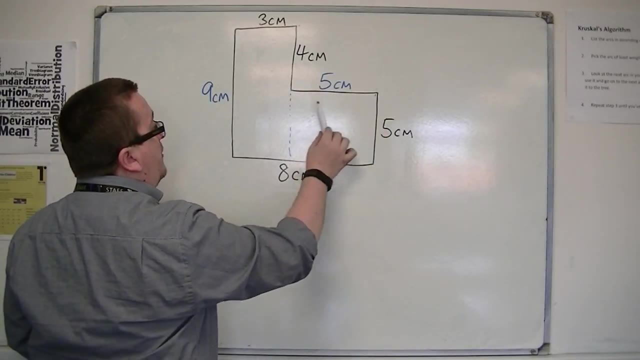 Each of them will give you the same area. I'm going to run with this one that I've drawn last. So we've got 5cm by 5cm. So this is actually a square. So this has an area of 25cm squared. 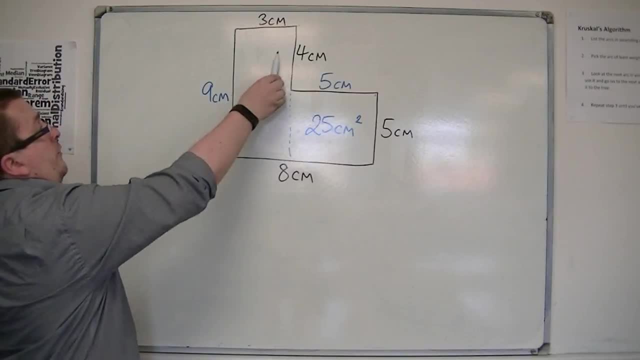 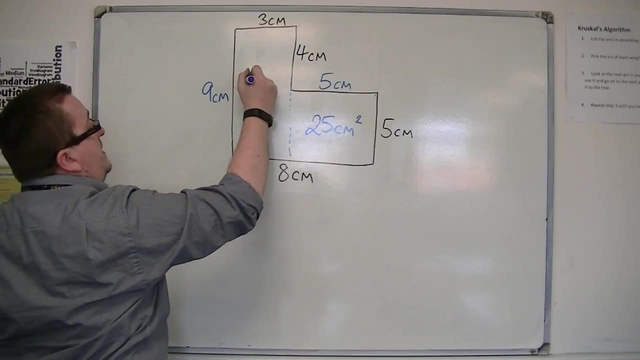 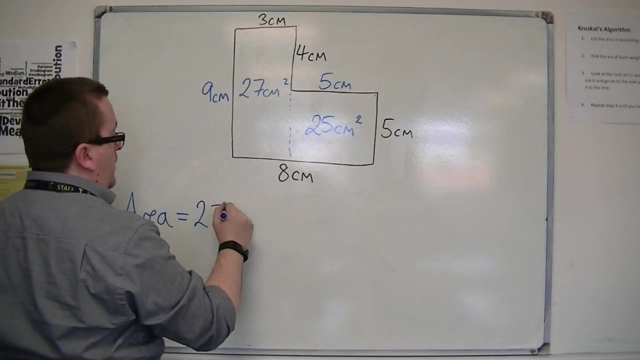 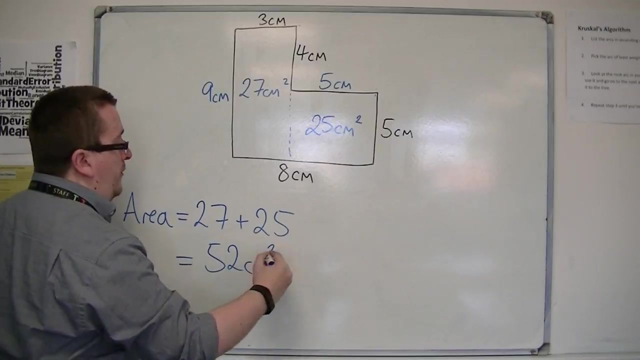 5 by 5. This rectangle is 3 by 9. So the area of this rectangle is 3 times 9. So 27cm squared. So the total area is 27 plus the 25.. Okay, So that gets me 52cm squared.